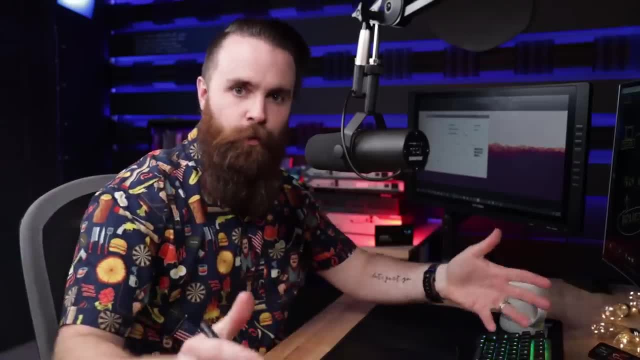 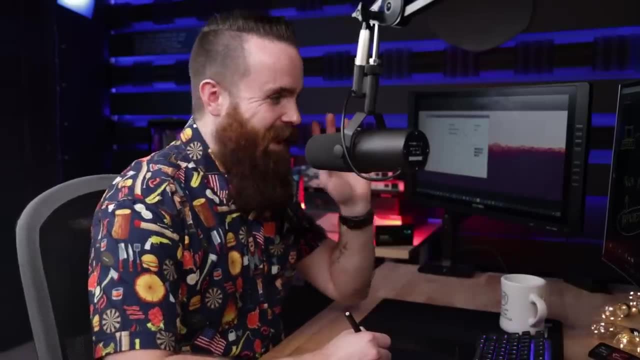 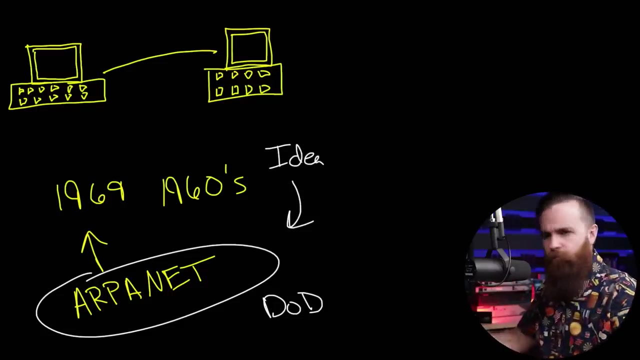 People could actually have their computers talk to each other, which I know sounds like not a big deal right now, but back then that was it. That was the new thing. But hold on, Here's the problem. though This was more of an idea, They legit did it. Here's the first network diagram. I think there. 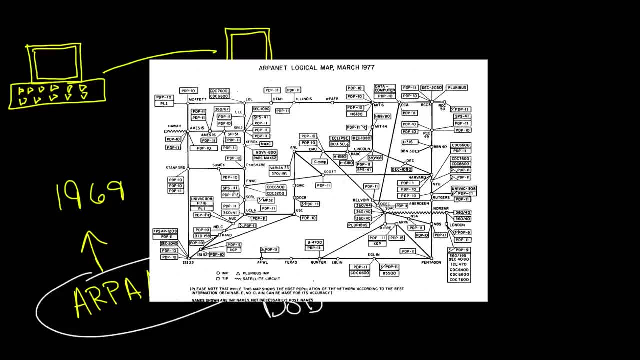 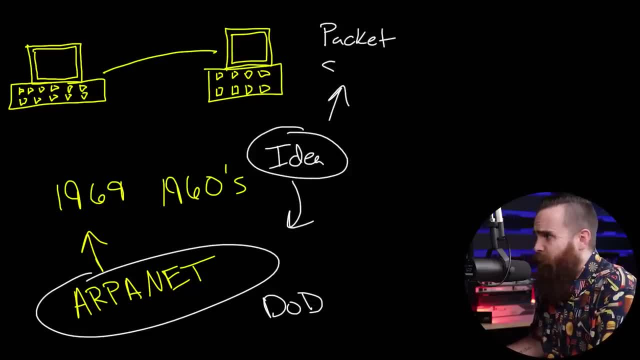 ever was Check this out. Look at that thing. I have no idea what's happening. And when I say idea, they were like, yeah, this is a cool thing we can do. They actually invented what's called packet switching, which is what we do today, But what they didn't have. 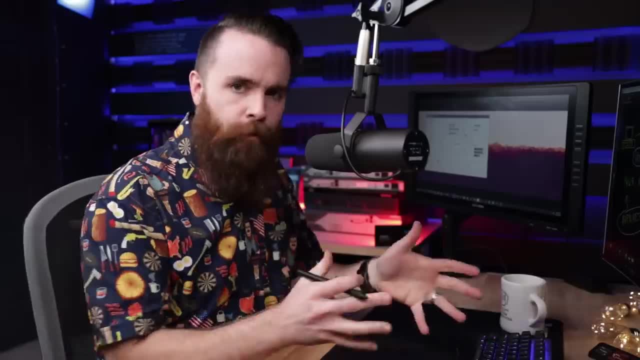 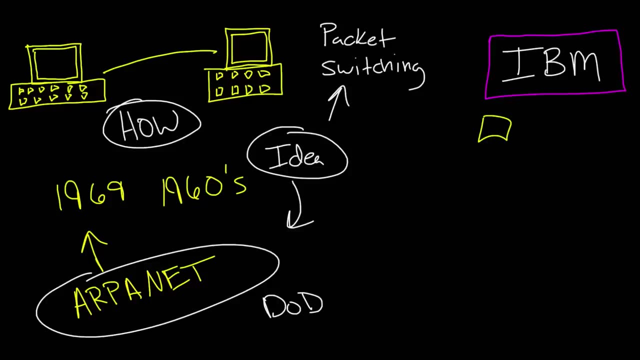 yet is the how? How do we make these computers talk to each other? You see, that part wasn't quite ironed out, But the idea, the idea spread like wildfire. So companies like IBM, they were like: heck, yeah, we have computers, Let's design our own network. And they did. It was. 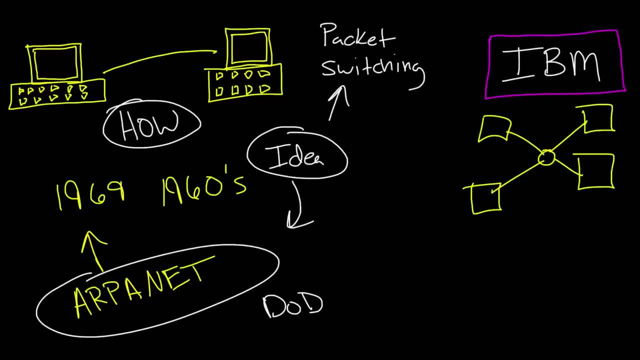 proprietary, meaning it only worked with their stuff, which is fine if you have an IBM computer. but there wasn't just IBM, There were other companies. And guess what these other companies did? They also designed their own networks. And I'm sorry, let me step back When I say design. 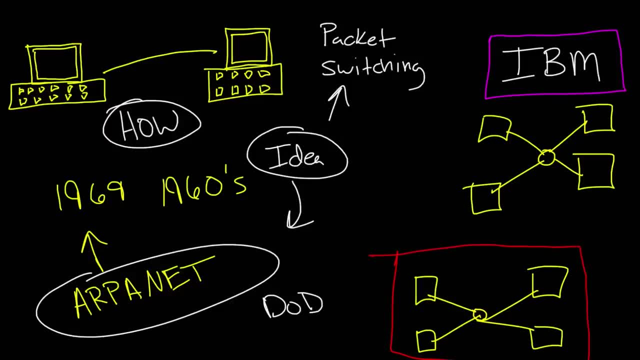 I mean they like, invented their own networks. They came up with the idea of how to actually connect computers together, And because these networks were proprietary, they couldn't really play well with others, meaning these networks could not communicate. You couldn't have this. 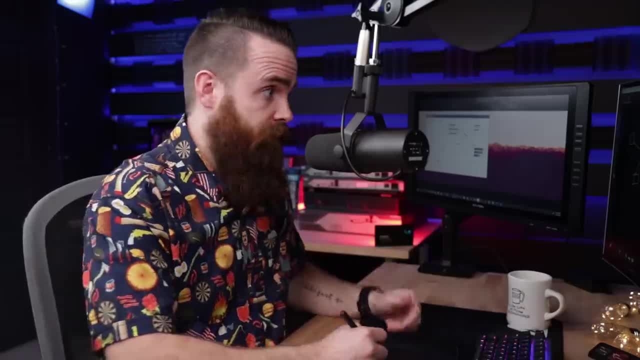 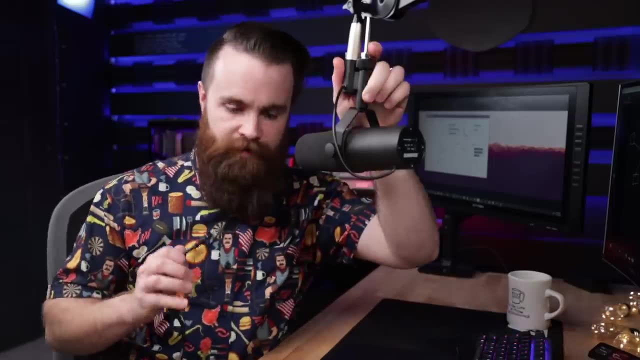 device talk with this device. They were basically speaking different languages. This network over here is like bonjour And this network over here was like what, No idea. Now I want to hammer this home, because this is some primitive stuff. I'm talking like. this is before ethernet cables were. 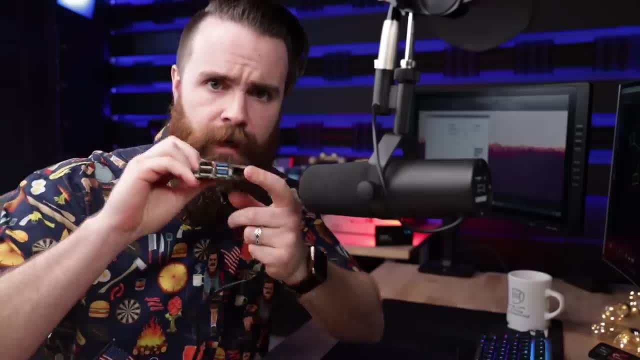 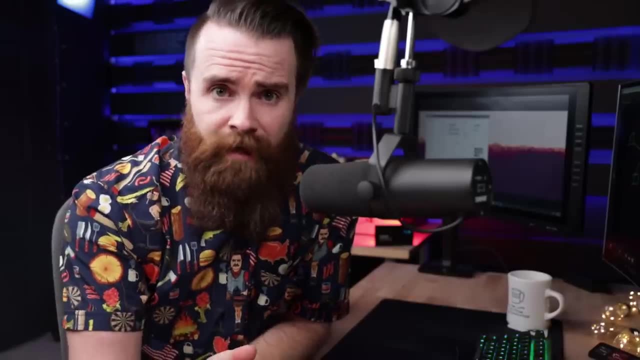 invented. Like we're so used to ethernet cables, We're so used to the ethernet ports, These weren't a thing. Each of these companies had different versions of what it was And they were like they called theirs. Like you ever try to charge your iPhone with an Android charging cable? 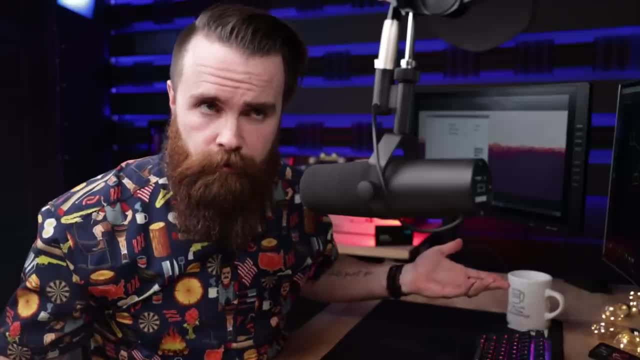 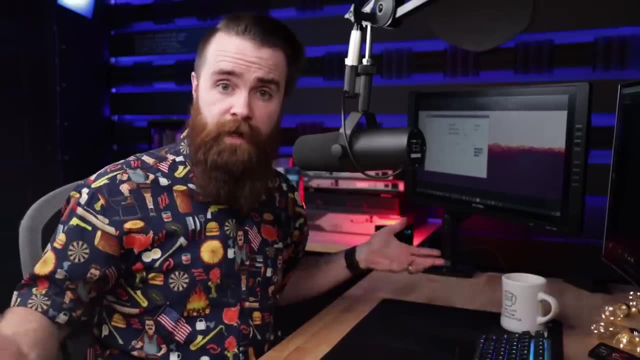 It doesn't work. It's just not compatible. That was the networks of yesteryear or long time ago. Now eventually they realized, Hey, this is kind of stupid. Maybe we should all use the same networking stuff. Yeah, let's do that Now. easier said than done, This involved 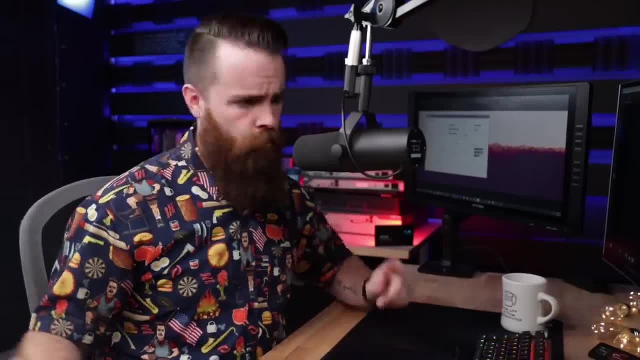 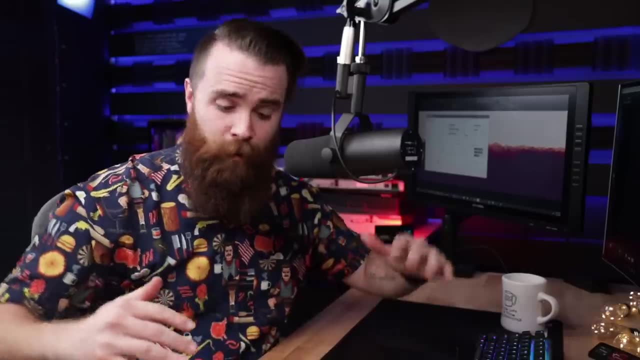 meetings and committees and I want to do this. I don't want to do that. You're wrong, sir- A lot of that kind of stuff. Now, there's a long and maybe interesting history, If you're into that, of how this all came about, but we eventually ended up with a networking model. 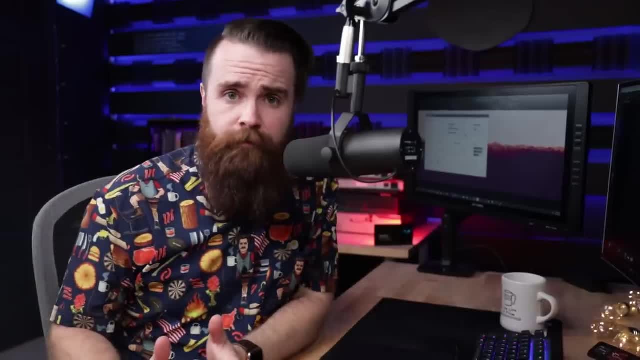 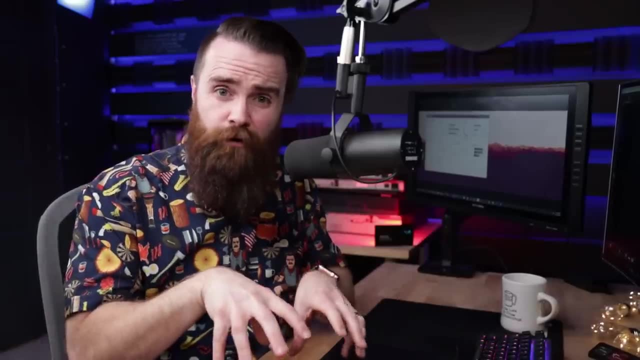 A model that defines how we can connect our stuff, So that when IBM makes a computer, when Apple makes a computer, when Microsoft makes a computer, we're all putting the same technology inside that computer to make it talk to the other computers. That's why it's such a. 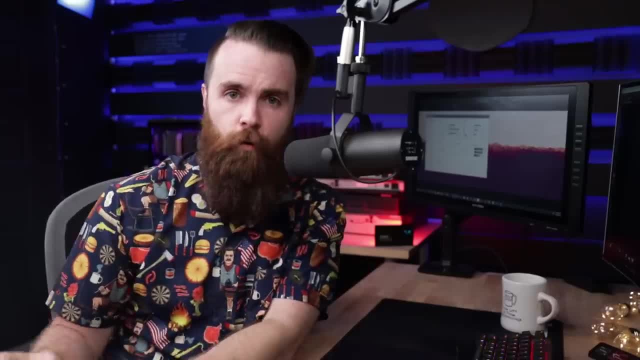 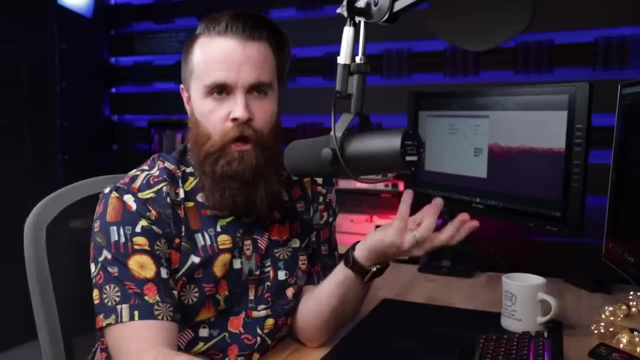 beautiful thing that a Microsoft computer can send a photo to an Apple computer. We're all using the same networking technology. We're using the same networking standards. Now, actually, honestly, we ended up with two models: one that we actually use And then one that we 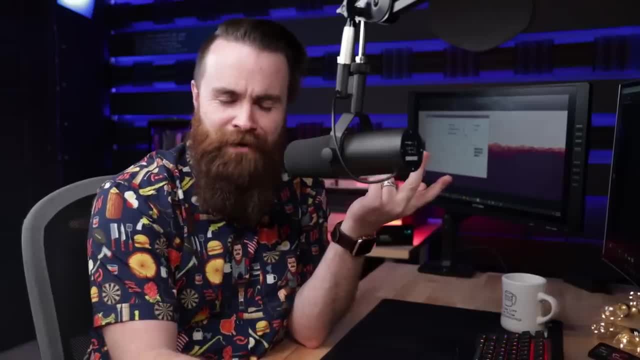 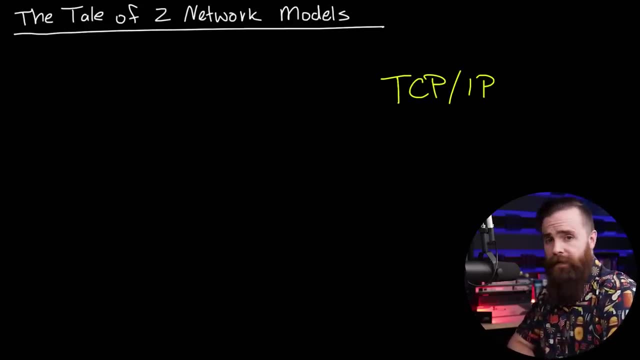 still cling onto and talk about all the time. I'll show you. the model we use today is called TCP IP. This is what every computer supports and has implemented into their system- the TCP IP model- And they also call it the TCP IP stack. Now the 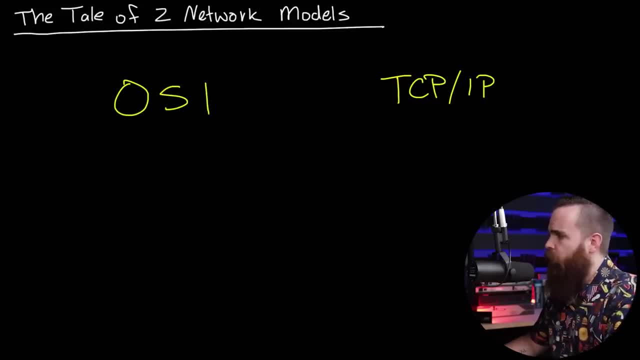 other model. he wanted to be the one that won so badly. People were on his side, They were campaigning, but he just did not win TCP IP one for a variety of reasons, but it was just more widely adopted. So then why am I still talking about him? If TCP IP one, I'll show you It's. 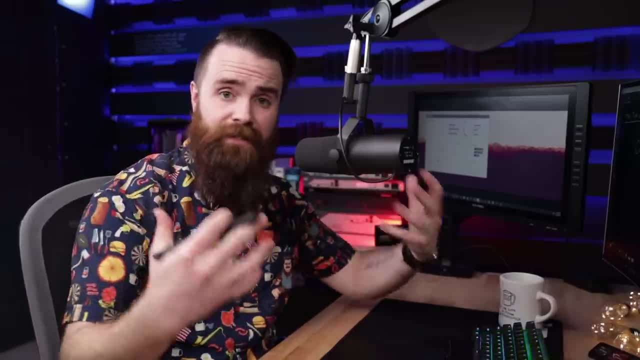 weird. Now again, TCP IP one is a model that we use today. It's called TCP IP one. It's called TCP IP: just a list of rules or guidelines, standards on how computers can communicate, how we design those systems, And there's a lot that goes into that. So to make things more simple, 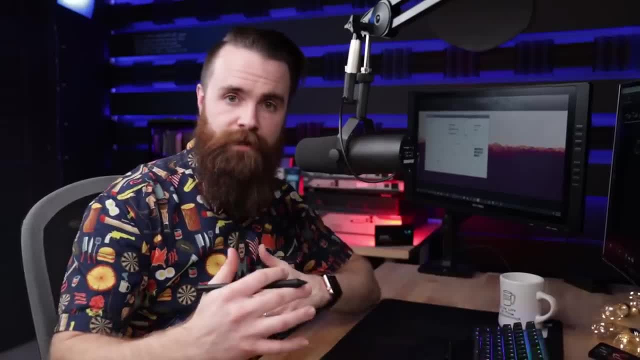 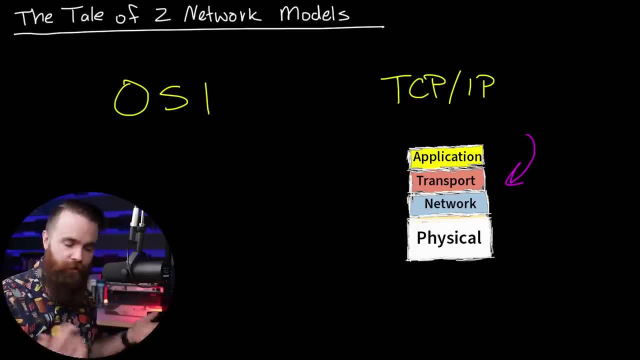 more digestible, easier to understand and implement. we divided all those functions into layers, layers like this right here. Each of these layers define some kind of protocol or standard we'll use when computers connect. So, for example, the physical layer. we know it's. 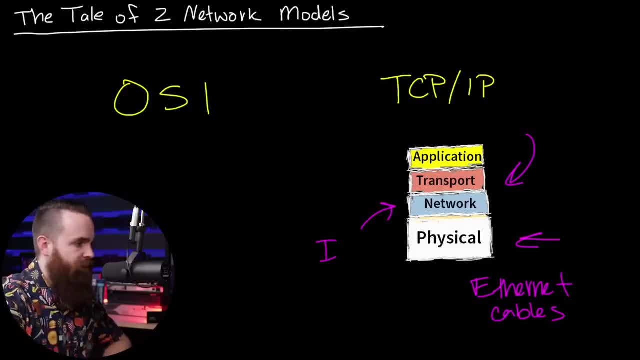 going to involve ethernet cables, the network layer, all about IP addresses and routers. So with this standard we all agree we're going to use IP addresses when we communicate over the internet. Before that standard that wasn't really the rule. You could have done anything You could. 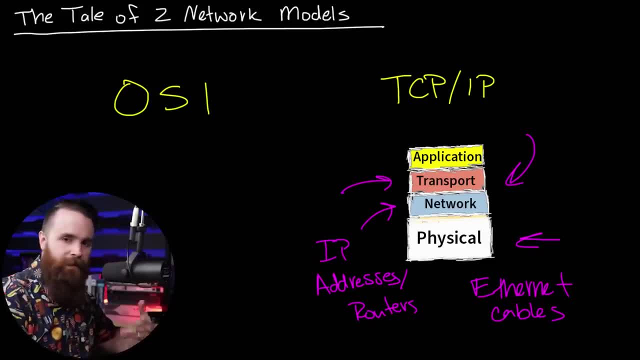 have used names from Star Wars or something I don't know. Transport: we got TCP, UDP port numbers. We'll talk more about that later. And then application: like hey, when I open up my web browser and I go to netflixcom, what protocol am I going to use? Do we all agree to use the same? 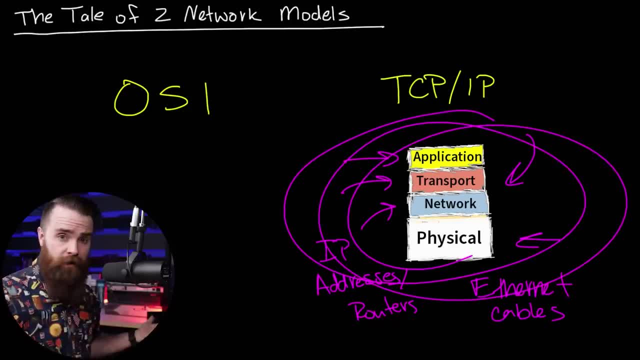 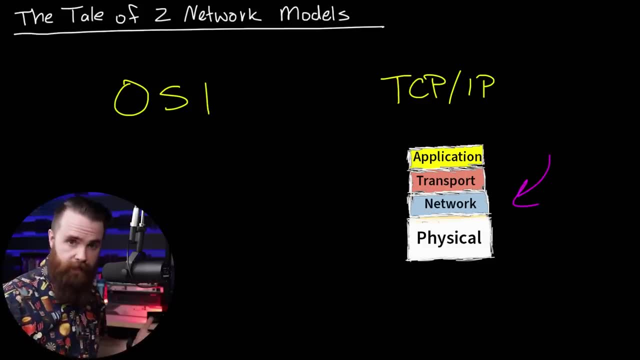 protocol. We all agree to use the same stuff and it's beautiful. Now we can all talk together, We can all network together. Now this is the traditional view of the TCP IP model, the layers we see here. If you're studying for the CCNA- the 200-301,, you might see the physical layer divided. 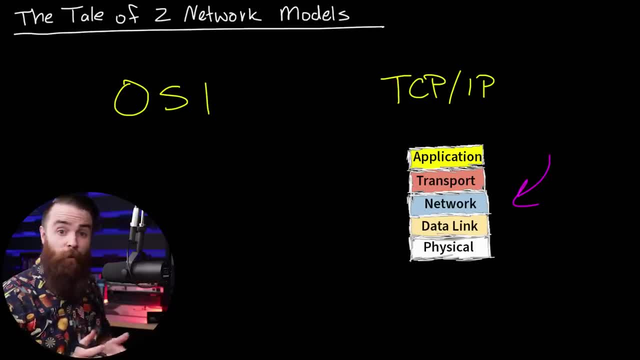 into two separate layers like this, which I happen to love, And if you watched my last two videos in the series, you're already familiar with the first three layers here. You've already seen them in action going through a network. We get our physical: the ethernet cables, the network cards. 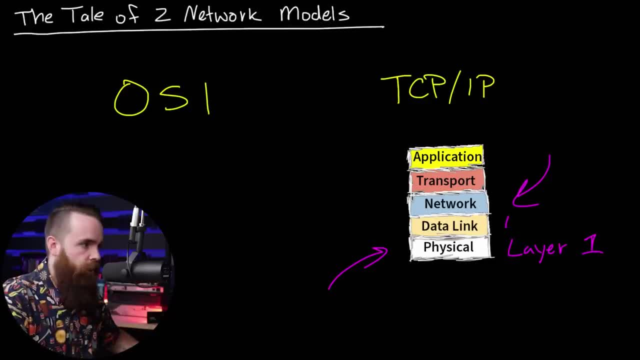 the electricity flying. That's our layer one. And then we talked about our data link layer. This is where our Mac addresses come in. our layer two addresses how hosts on the same network can communicate And the switch uses those layer two addresses. And then we talked about the 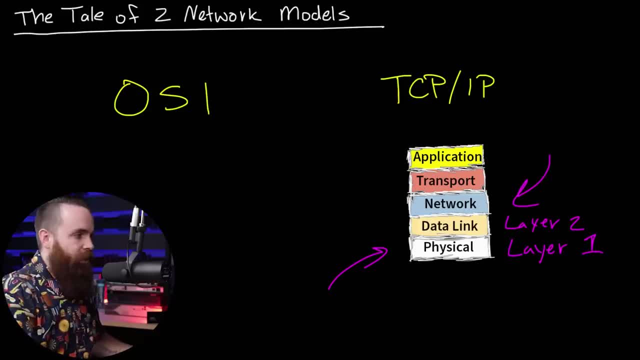 those Mac addresses to know where to send information. And then, of course, we have our layer three, our network layer. We know this to be IP addresses. We know that we assign our devices IP addresses and this is how they communicate. This is how the router can know where to find. 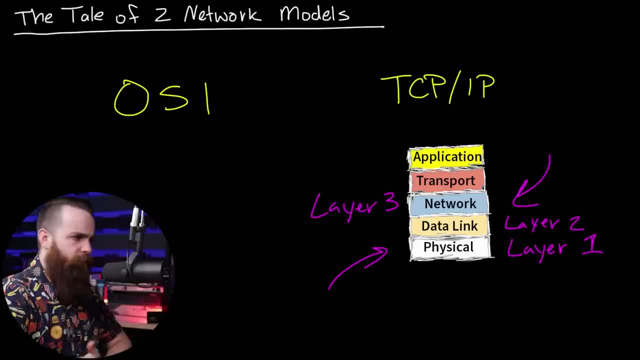 people and route those packets to the right people. And then we have our other layers and we will talk about those, but not right now. We'll get to it. Okay. Now what about the OSI model? Where does this guy come in? Well, let me show you. Similar to TCP IP, he works on layers In. 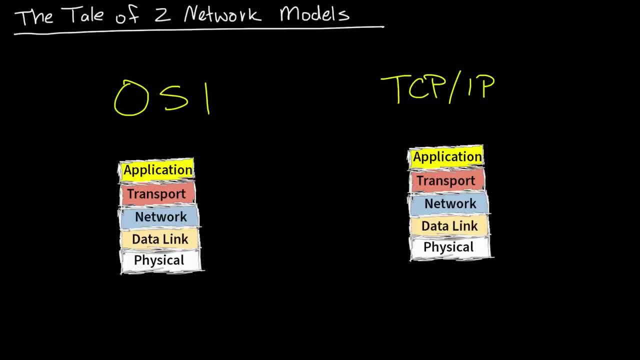 general, he just has a few extra. So physical data link and network transport, Yeah Yeah, Let's talk, That's the same, But then at the application layer it's a bit different. We're going to add a couple more. We're going to add a session layer and a presentation layer. Let me scoot this guy. 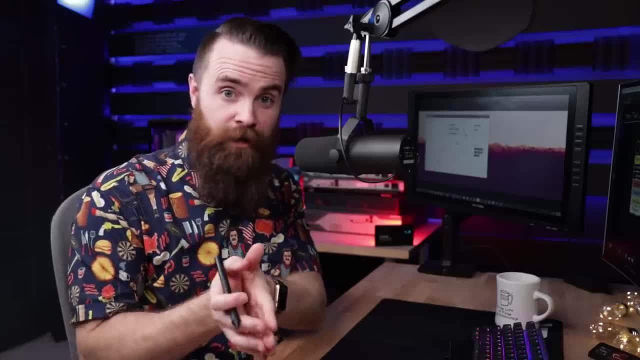 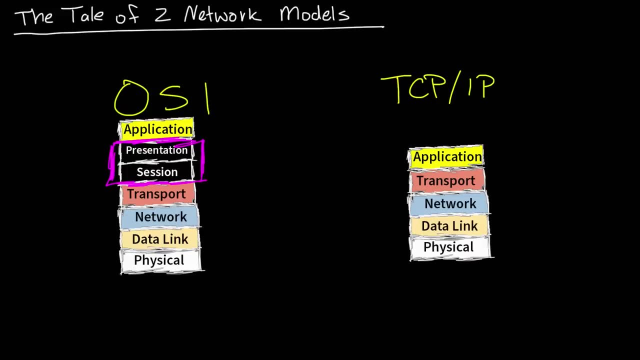 up a bit. There we go Now. as you're studying networking as a network engineer, the main difference between the TCP IP model and the OSI model are these two extra layers. Now the concept of these layers, what they bring to the table. do not go away with the TCP. 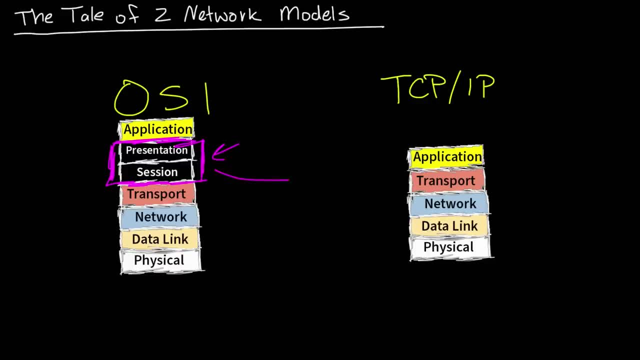 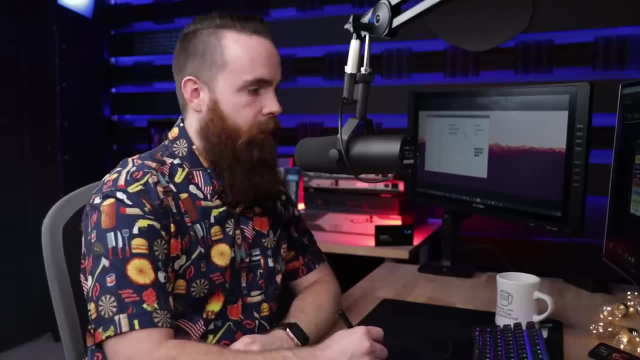 IP model. I'm saying it too much. All that happened is we stuffed those two layers inside the application layer. but, Chuck, you still haven't told us why we're talking about the OSI model. Why are we even talking about it? This is why I told you these two models were at war. 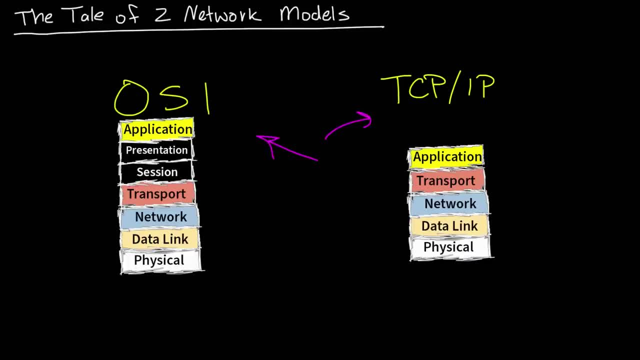 with each other who is going to win, And during those wars, it was widely believed that the OSI model was going to be the one that was adopted- which, by the way, stands for open systems interconnect- And because it was thought to be the clear winner, we started using the layers that the 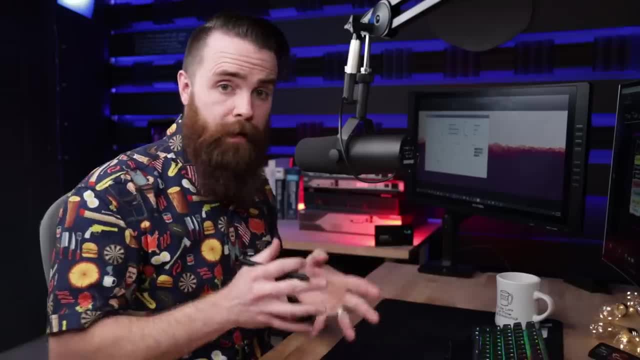 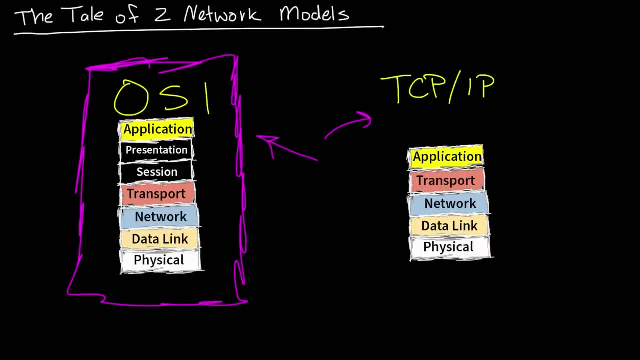 OSI model has as our day-to-day terminology And even when TCP IP models were at war with each other, TCP IP was the clear winner and it killed and murdered OSI. We still refer to the OSI layers when we describe network functions. Now, again, not a huge deal, because layer one, two, three, 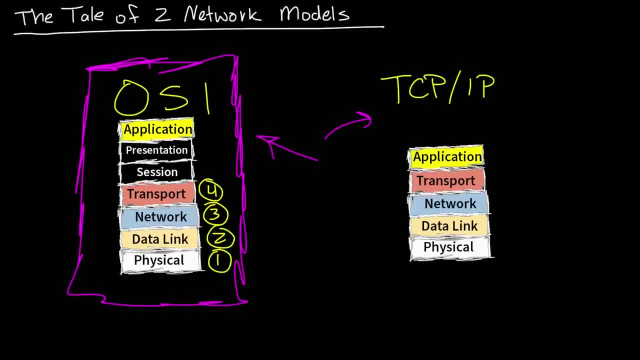 and four are the stinking same as the TCP IP model, as long as you're referring to the Cisco version of it right now. But when you get up to the layer five, layer six and layer seven, clearly we got a little disconnect there. But when network engineers talk about it, OSI always wins. 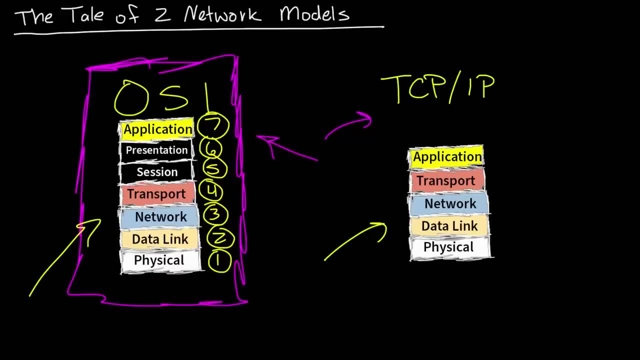 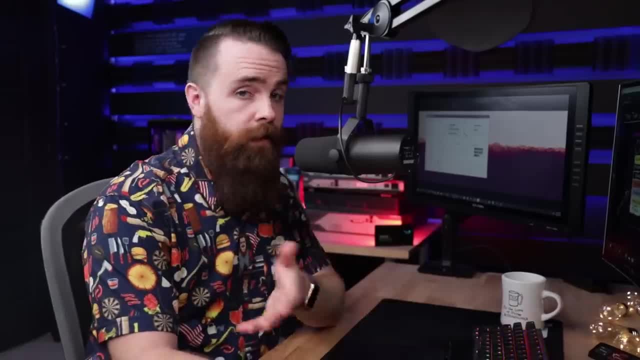 We will always, always, always, refer to the application layer as layer seven. This right here is layer seven, And there's only five layers here. That's just how we do it. That's how we roll. But I will say this: If you're trying to learn networking, if you're studying for the CCNA, you need to know. 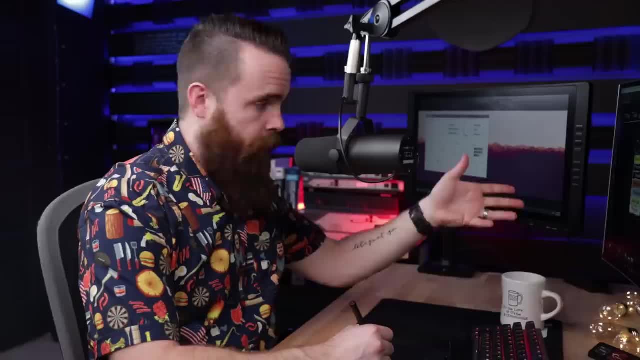 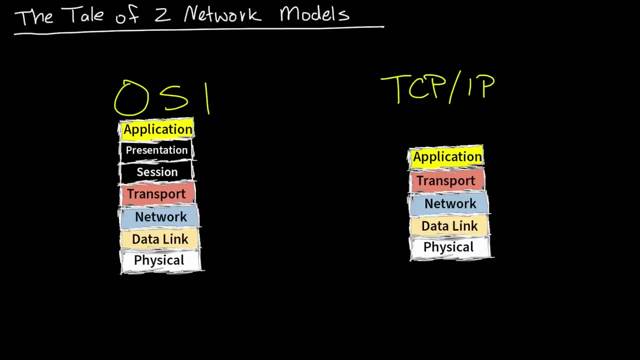 both of these models. There's a fun way to memorize this. So the OSI model seven layers, harder to memorize. We'll use a mnemonic device. So application presentation session: transport network data link- physical, Let's try. all people seem to need data processing, I'm sure. 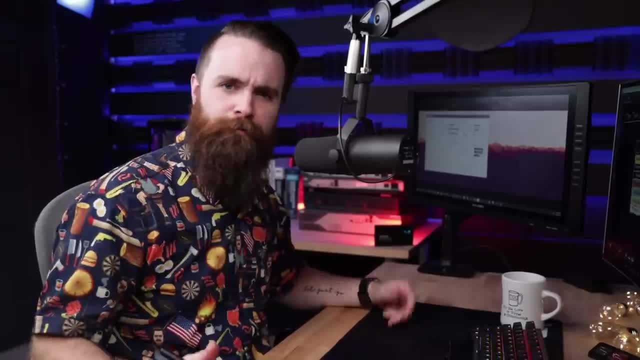 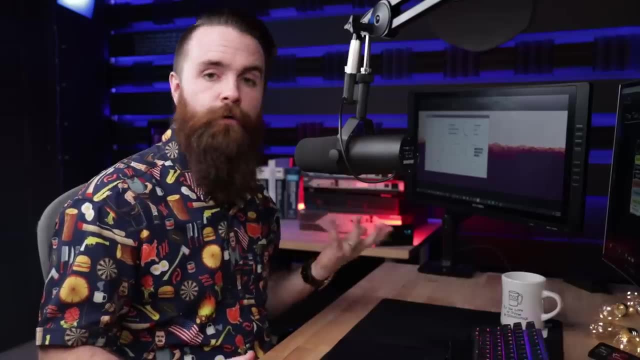 there are better ones. That's just how I learned it. Let me know below if you have a better one. I can't tell you how many times throughout my career I've referred to that phrase, that mnemonic device to remember the seven layers. And then what about? 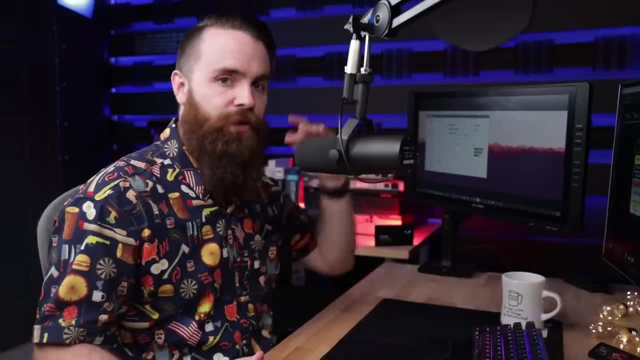 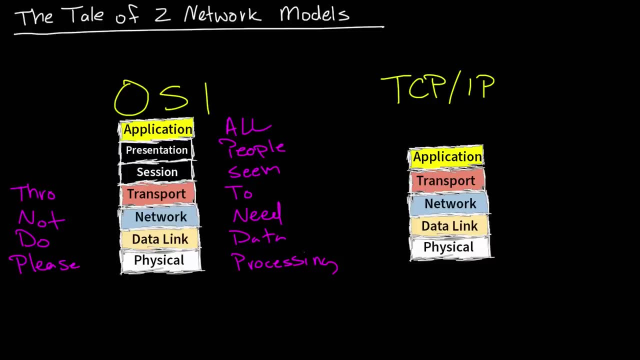 reverse. What if you're not going from application to physical? What if you're going from physical to application, which can happen routinely? right, I got one for that too. Please do not throw sausage pizza away. Makes me hungry every time. Now, again, a big reason to remember and memorize. 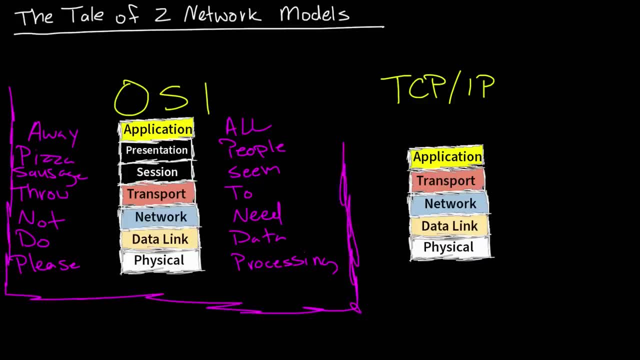 the OSI model is: A- you need to know it for any exam you might be studying for- And B- it's honestly the thing we reference the most when network engineers are troubleshooting or working through any kind of networking issue. Oh, that's a layer seven issue application. 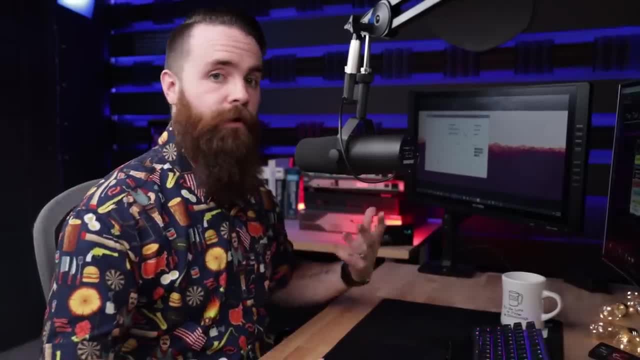 Hands off, not my problem. Or hey, that's a layer one, layer two, layer three or layer four issue. Okay, time to see what you learned. Get your copy ready, your thinking cap on. Let's do this Exam. 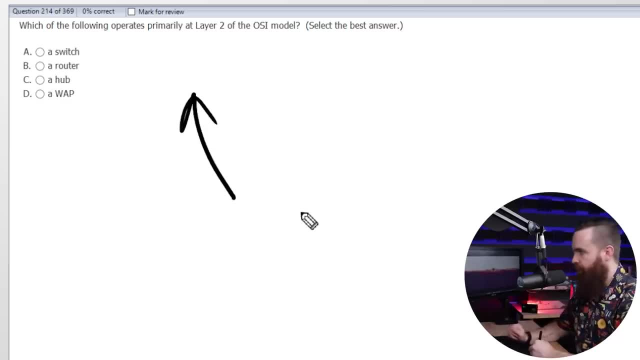 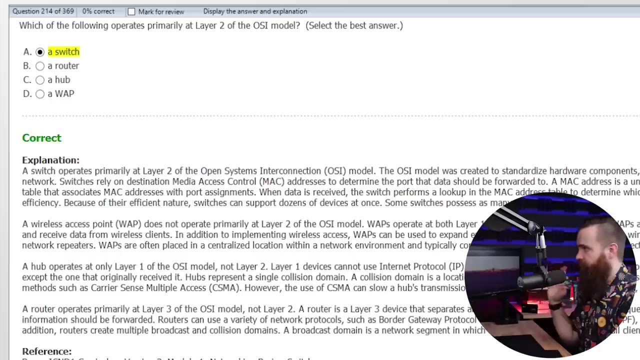 questions right now. Question number one: which of the following operates primarily at layer two of the OSI model? Select the best answer And go. If you said the answer was switch, you're absolutely right. If I hit show answer fingers crossed: Yes, I'm right, The switch. 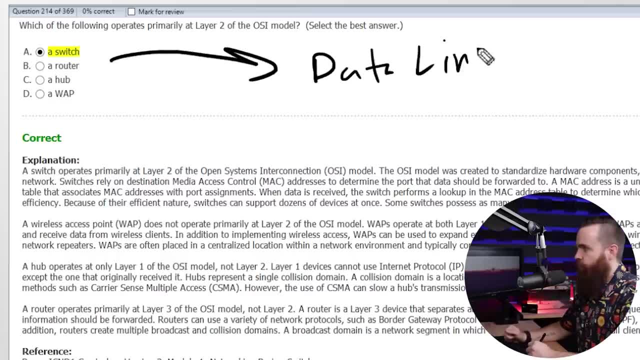 operates at the data link, layer layer two of the OSI model Router Nuh-uh. Where's the router? operate at Layer three IP addresses, the network layer, The hub. That might've been a little bit confusing for you, because we compared switches and hubs in one of our earlier videos in the series. 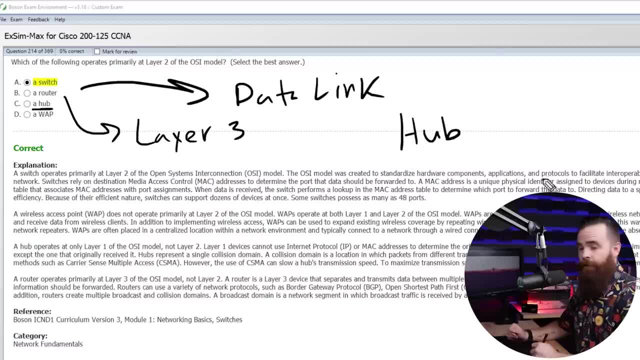 Where do they operate? Remember, hubs are stupid. They got no smarts. They don't operate at layer two. They're not even aware of Mac addresses. All they do is use the OSI model. They don't know the OSI model, They just repeat electrical signals when they receive them Out all ports. So they are. 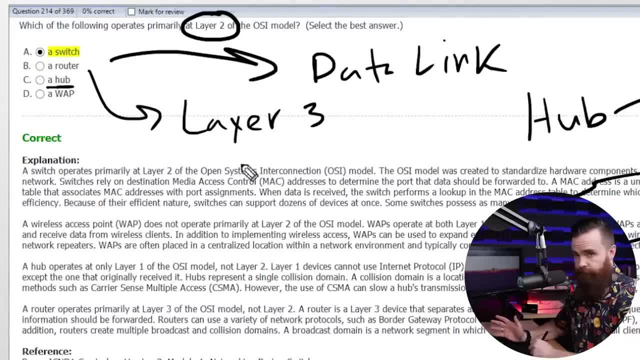 primarily physical And quiz what layer is physical? Layer one right, And then a WAP, a wireless access point. This was kind of a tricky one, because they do operate at layer two. They also operate at layer one, So they're not primarily focused on layer two. So if you put 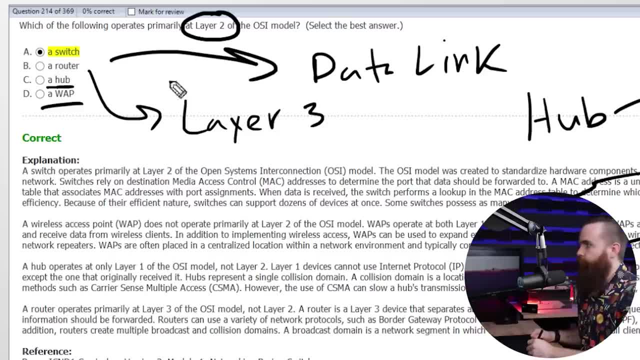 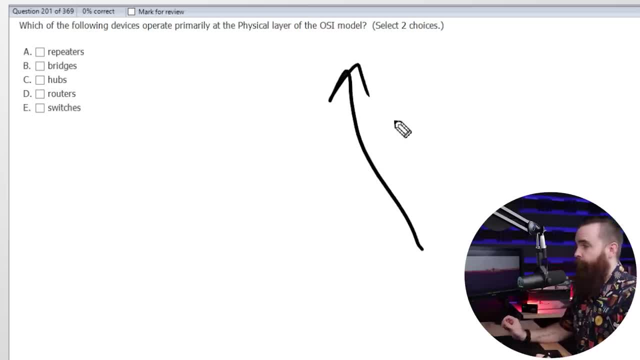 that answer. you're half right, You're kind of right, But we're looking for what primarily operates at layer two, And that, of course, is a switch. Question number two: which of the following devices operate primarily at the physical layer of the OSI model? Select two: 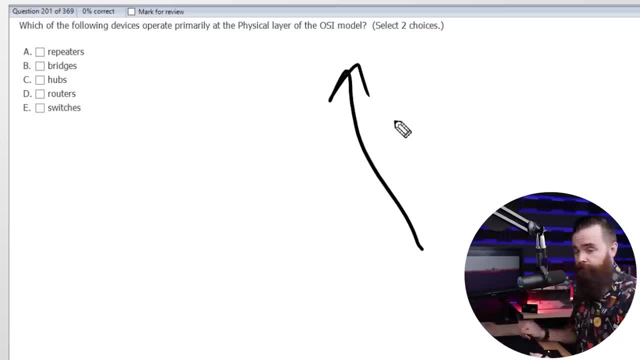 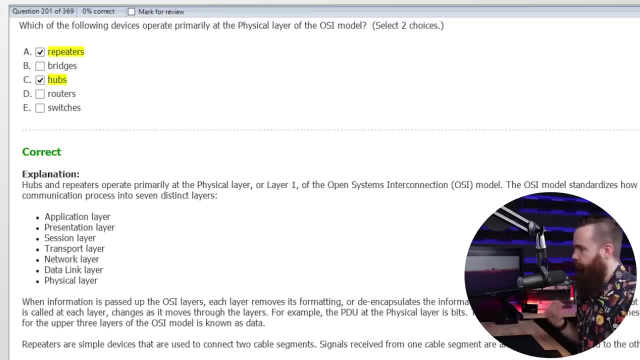 choices. Now we kind of already covered this. Let's see what you got Go. Okay, here we go. Here are the answers: A repeaters And C hubs. Let's see if I got it right. Boom, Now this may. 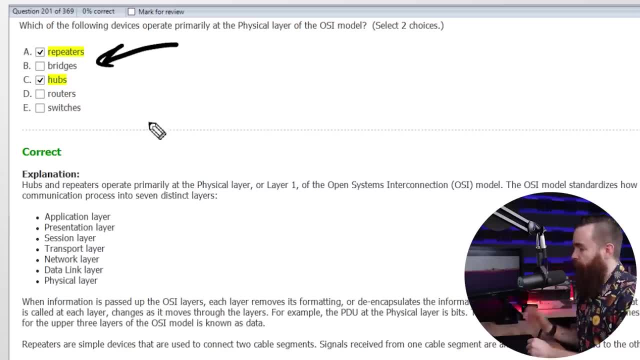 have been a bit tricky for you because we haven't talked about bridges, And that's fine. But through the process of elimination we know that. hey, switches, those are layer two, And we just talked about that. Routers, layer three, of course. We just said that hubs are physical And I even 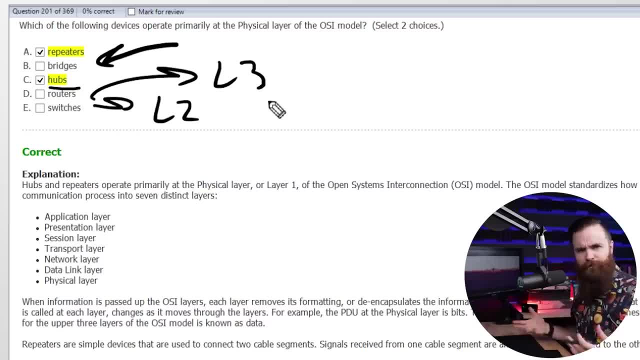 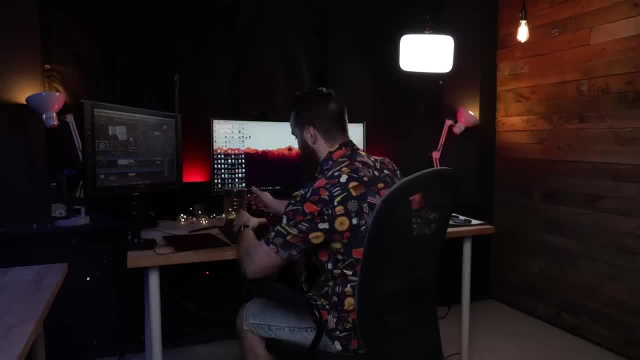 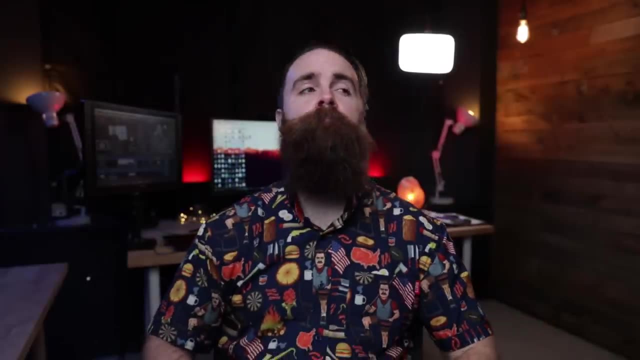 repeat electrical signals when they receive the electrical signals over the wire, And repeaters do the same thing. Bridges, on the other hand, are similar to switches in that they do deal with layer two. Well, guys, that's about it. If you like this video, hit that like button, If you. 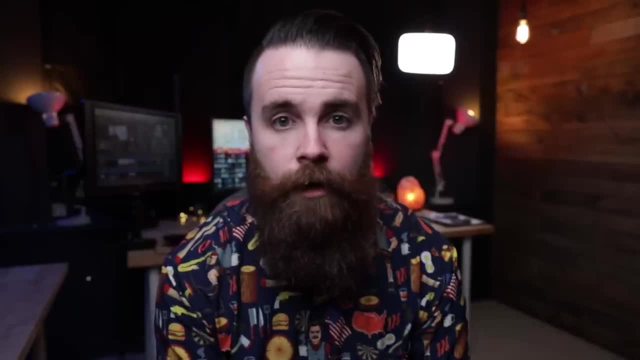 have any comments or questions or need help with your CCNA. comment below Or you can jump into my Discord server. A ton of guys in there, a ton of gals in there helping people with their stuff, And I'll see you guys in the next one. 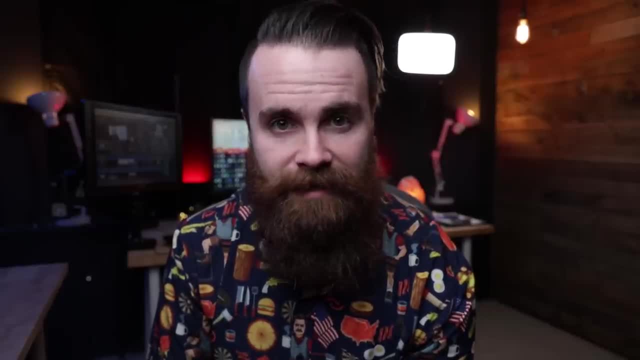 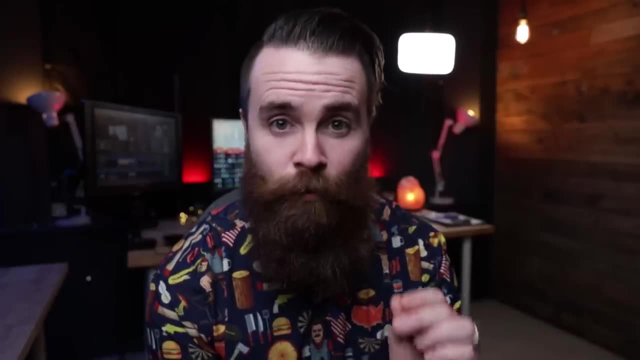 Now, if you want to see more of this, more stuff like this, go check out thisisitio. It's a membership that David Bombal and I run. Go check it out. It's pretty cool. And also, in just a few hours, I'm launching episode four of this series, where I dive deeper into 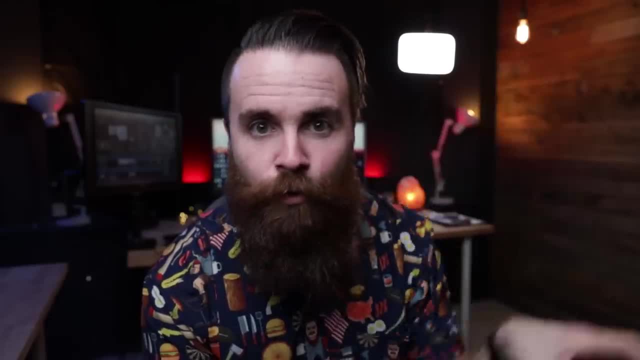 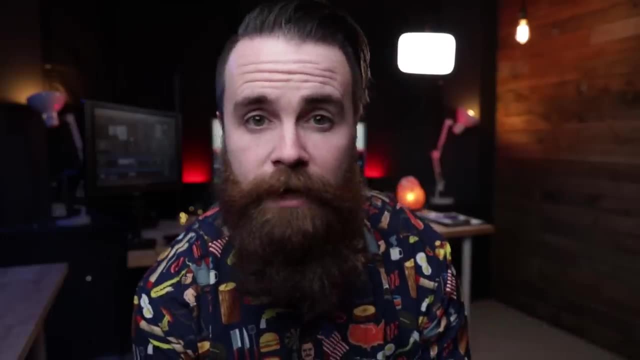 the OSI model and the TCP IP model, and we'll actually watch a packet go through a network and we'll analyze each layer as we hit it. So be looking for that. It already might be out actually, So check it out. Well, anyways, episode three. that's a wrap. I'll catch you. 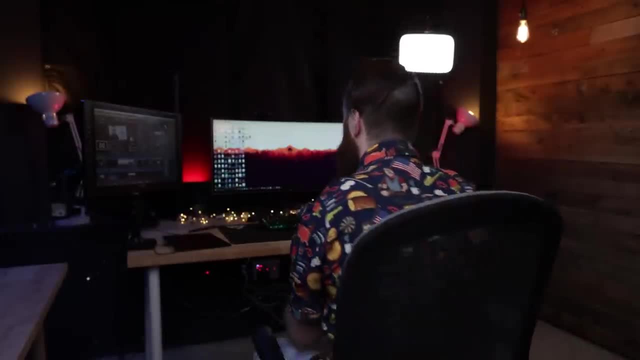 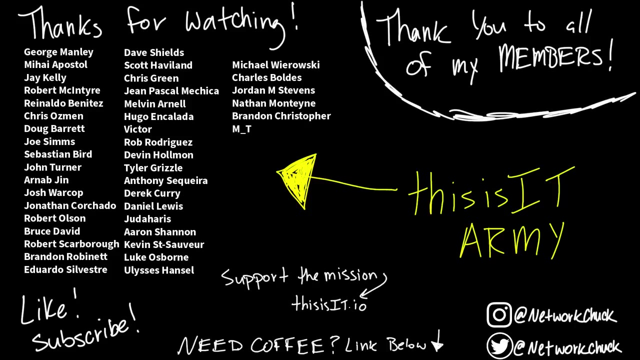 guys later. Bye for now.